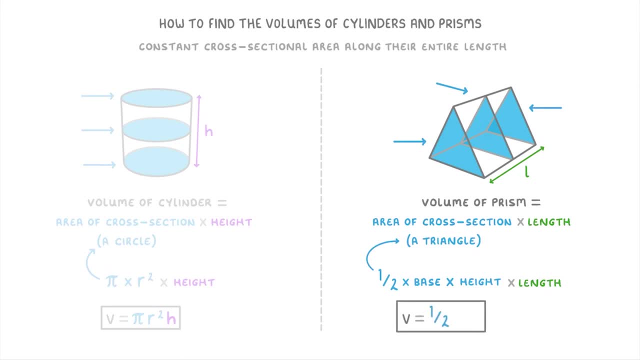 And we can shorten that one to volume equals one half b, h, l. To see how these formulas work, we can use the formula for cylinders, For example. if a cylinder has a radius of 3 cm and a height of 12 cm, we can add some measurements to. 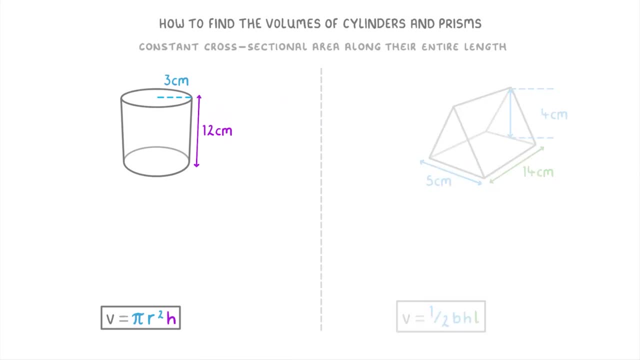 our shapes and calculate their volumes. So for the cylinder, we can see that it has a radius of 3 cm and a height of 12 cm. So to work out the cross-sectional area of the circle, we'd do pi times the radius of. 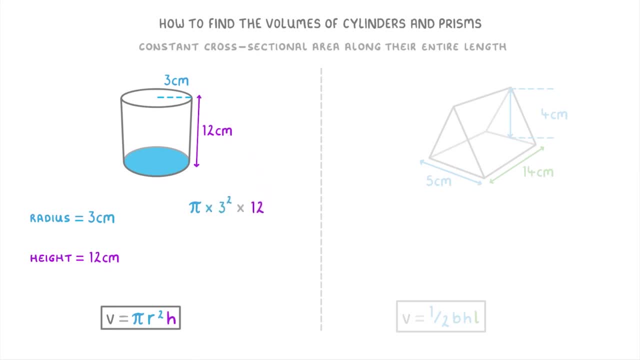 3 squared, and then we'd multiply that by the height of 12, which, if we wanted, our answer in terms of pi would be 108 pi cm3, because that's the radius of the cylinder. So we'd do pi times the radius of 3 squared, and then we'd multiply that by the height of 12, which 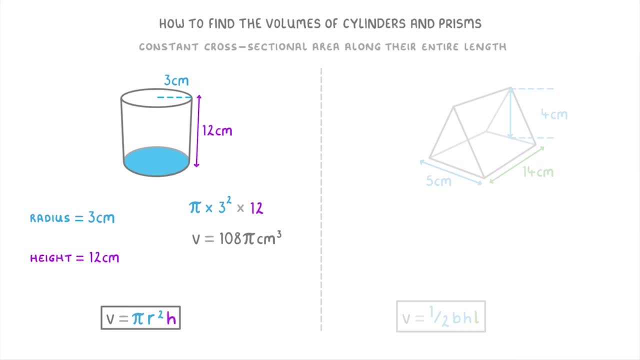 would be 108 pi cm3.. Then for the triangular prism, we can see that it has a base of 5 cm, a vertical height of 4 cm and a length of 14 cm. So to work out the cross-sectional area of the triangle, we'd start by doing one half. 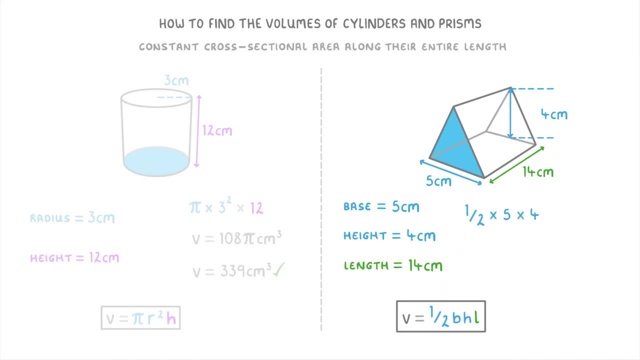 times the base of 5 times the height of 12 cm. So to work out the cross-sectional area of the triangle, we'd start by doing one half times the base of 5 times the height of 12.. So to work out the cross-sectional area of the triangle, we'd start by doing one half. 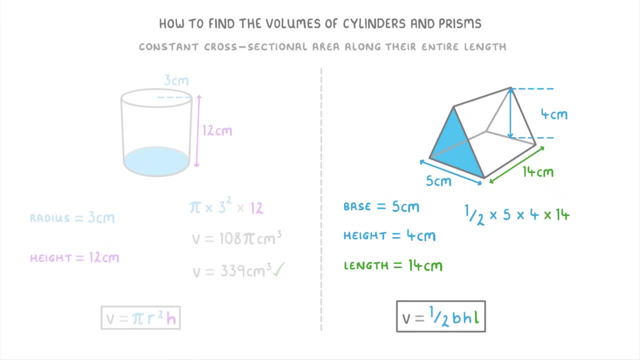 times the height of 12, which gives us a total volume of 140 cm3. And then we'd multiply that by the length of 14 cm, which gives us a total volume of 140 cm3.. One last thing to mention is that there are loads of other types of prisms as well, like 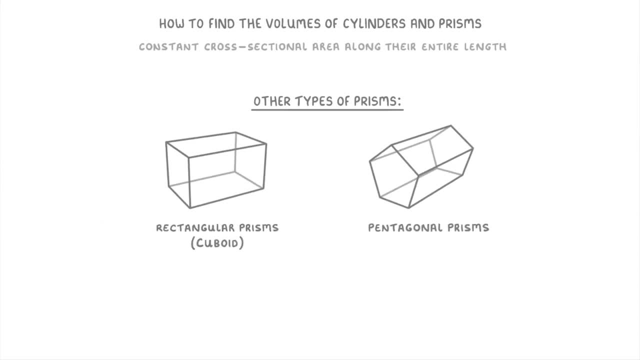 rectangular prisms, which are also known as cuboids, and pentagonal prisms, which have pentagons at either end. Whatever type of prism it is, though, the formula of volume prism equals area of cross-section times length will always work. It's just how you find. 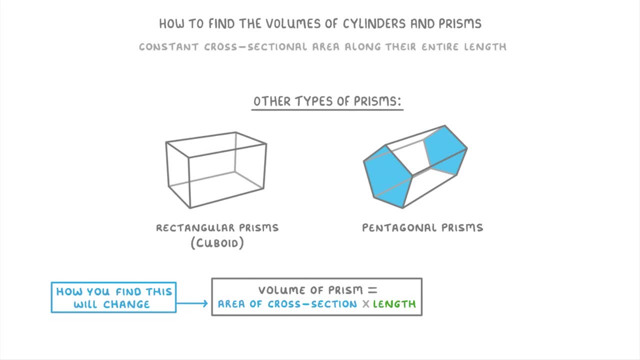 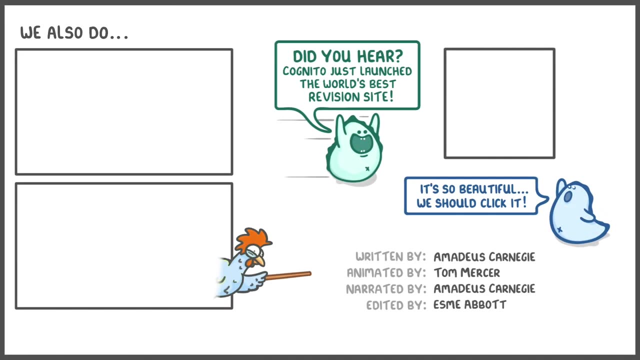 the area of that cross-section that will change between different types of prisms. Anyway, that's everything for this video. So if you want to practice questions on this stuff or anything else in science or maths, then head over to our platform by clicking. 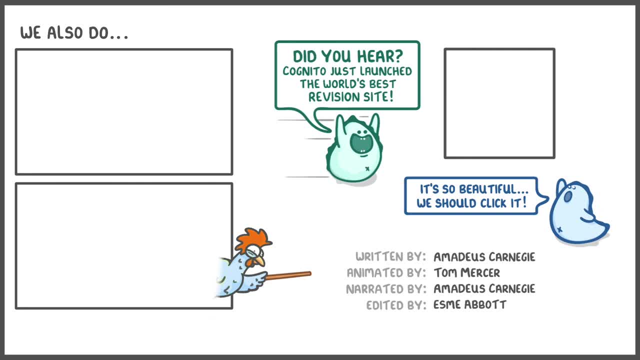 the link in the top right corner of the screen and we'll see you again next time.